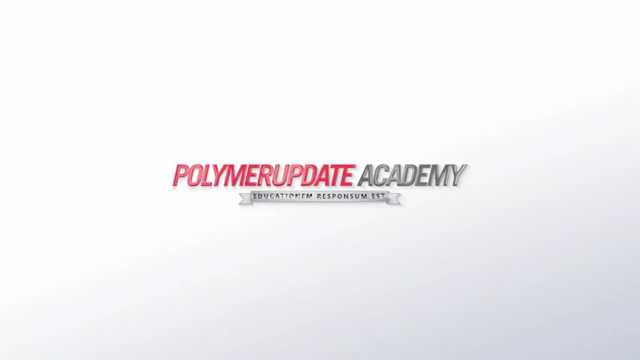 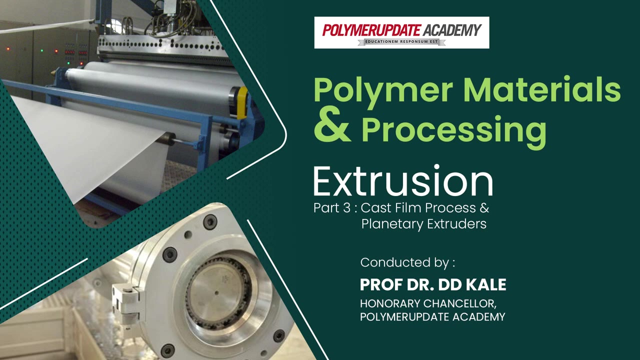 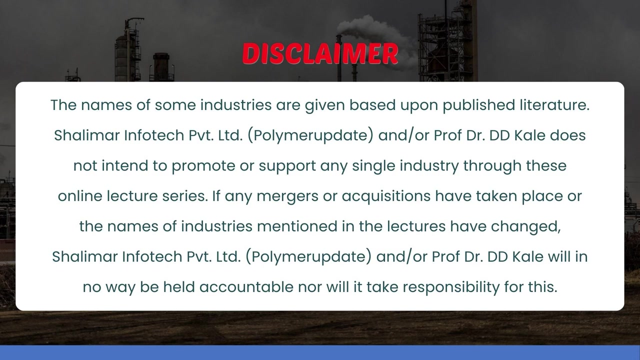 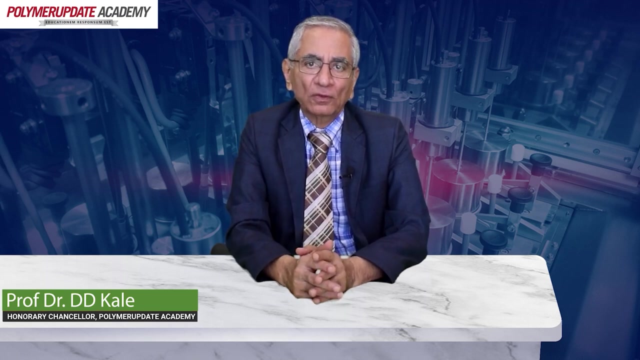 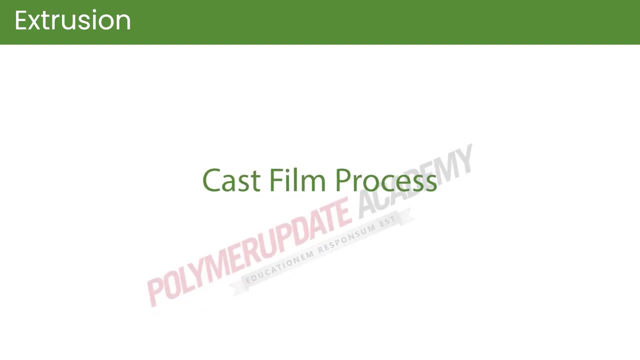 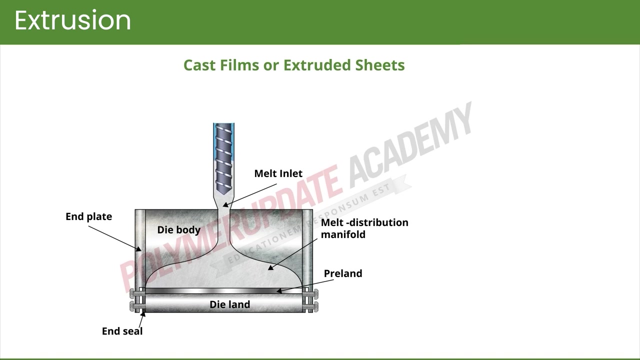 Hello everyone. now we shall see today the extrusion, which is one of the most important operation in polymer processing. Now let us look at the cast film process. The polymer melt comes out of the extruder, which is in a circular opening, and then the melt has to come out in the form of 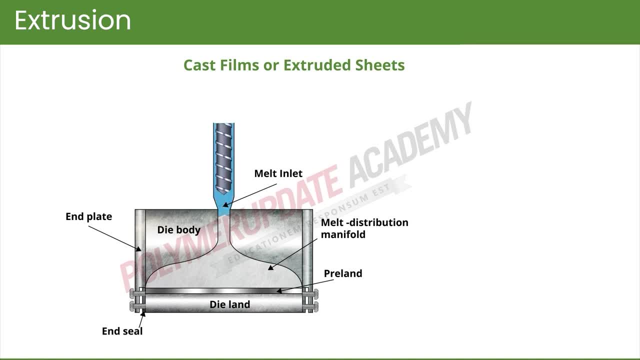 a thin sheet. Therefore, the melt flows between the two plates, which are separated by a very small difference. These plates are arranged in the fashion like a hanger die. The slow expansion of the die ensures that the melt flows smoothly from the outlet of the extruder up to the outlet. 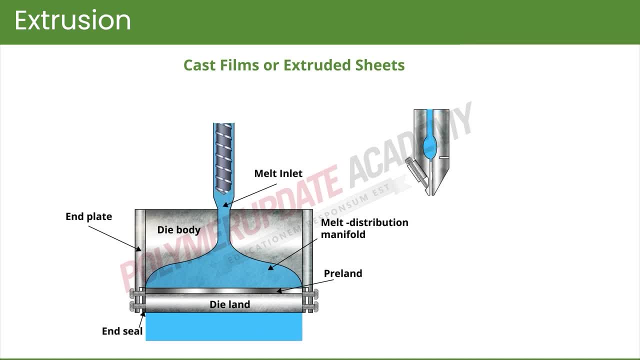 of the die. The outlet of the die is like a very thin layer of polymer melt. This polymer melt in a very thin fashion, in a very thin sheet like a structure, falls onto the chilled roller. The roller temperature may be of the order of minus five degrees centigrade or so. 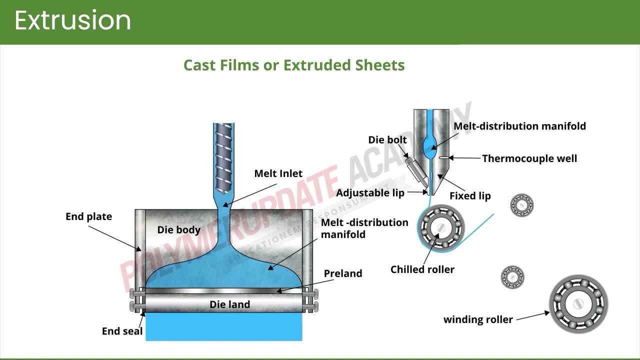 So as soon as it comes in contact with the polished surface of the chilled roller, the film gets completely cooled by the time it gets exit from the chilled roller. After that there are guide rollers and then it gets wound onto the winding roller and then it is processed further. 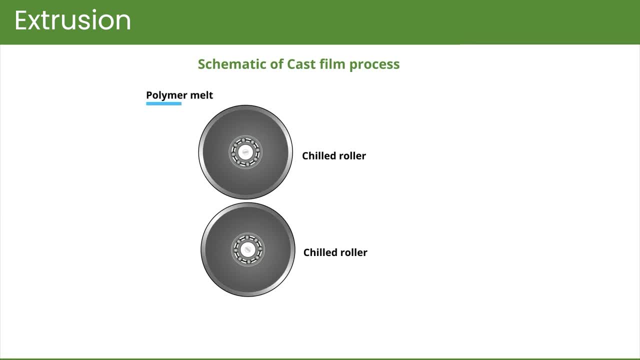 Another way of looking at it: chilled roller polymer melt is falling onto the chilled roller and it goes between the two chilled rollers so that film gets cooled very rapidly. and the film is completely cooled So as soon as it comes in contact with the polished surface of the 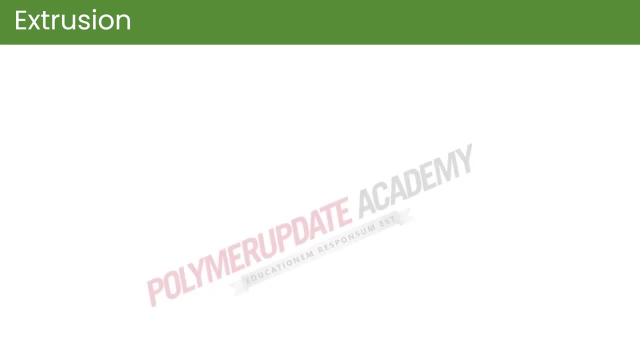 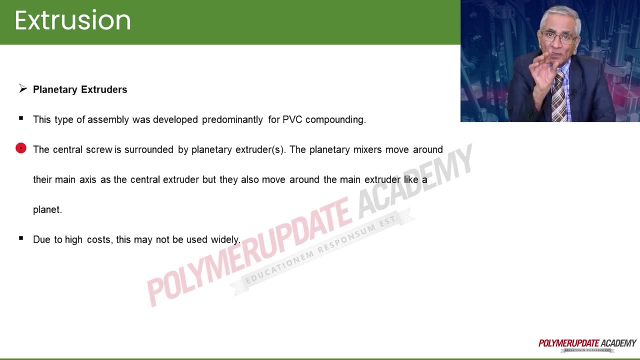 chilled roller. the film gets cooled very rapidly, and the film gets cooled very rapidly and what one gains is transparent film. Now we can go for planetary extruders. This type of assembly was developed predominantly for PVC compounding. The central screw is surrounded by planetary extruder or 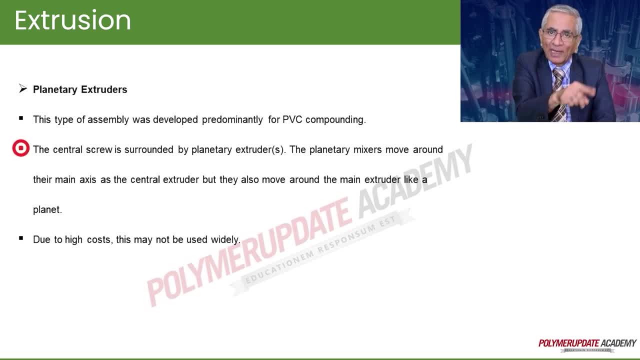 extruders. Planetary mixers move around their main axis as well as the central extruder, but they also move around the main extruder like a planet. Due to high cost, this may not be used widely. Now let us look at the schematic of planetary extruders. Many times they are often used to.